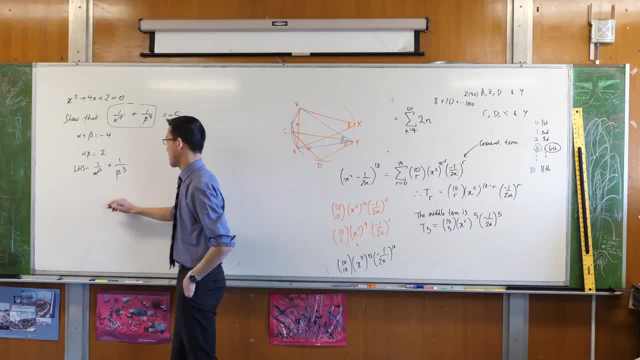 So when I think about how these things are going to go together, I think when I see a pair of fractions, my instinct is to get common denominators and combine them into one fraction. So let's go ahead and do that. If I multiply this by beta-cubed on beta-cubed, I'll get this right. That's that one. 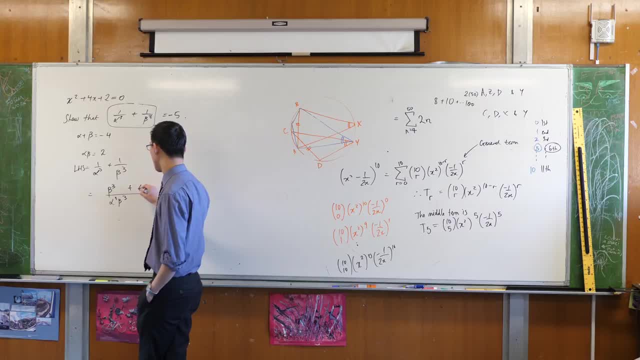 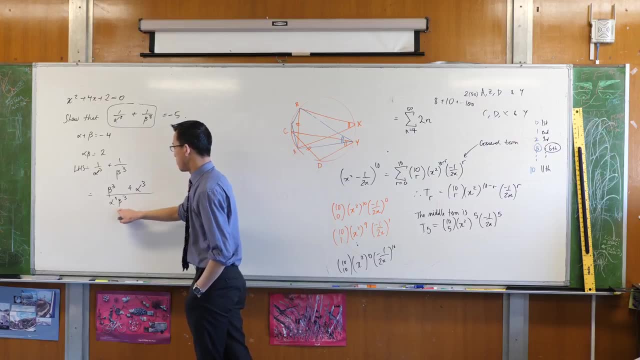 And then if I multiply this by alpha-cubed on alpha-cubed, I'll get this on the same denominator. Is that okay? Now, before I move any further, this thing down at the bottom I can work out directly, because something cubed times something cubed, is this all cubed? 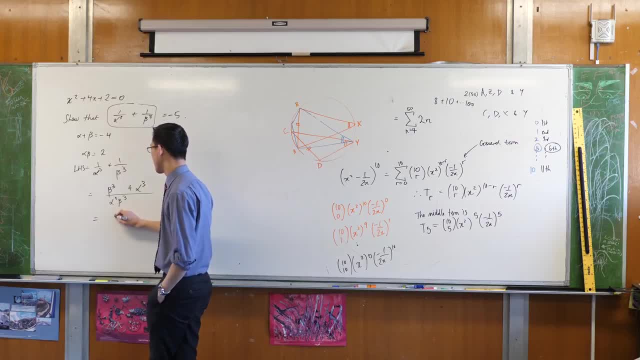 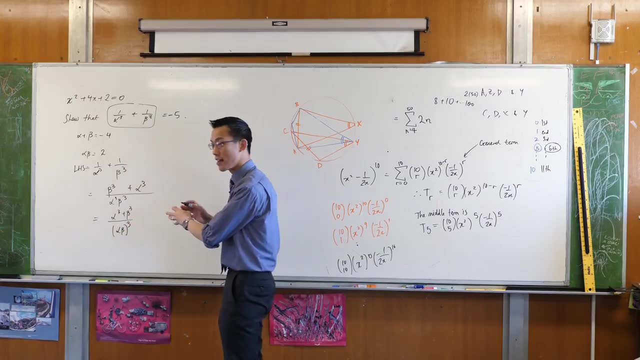 Do you agree? So I can use that. I will rewrite the bottom like so: Now this is just me mentally filing away. Okay, I know what to do with that, All good. But then you come to the top and you're like: what am I going to do with this? 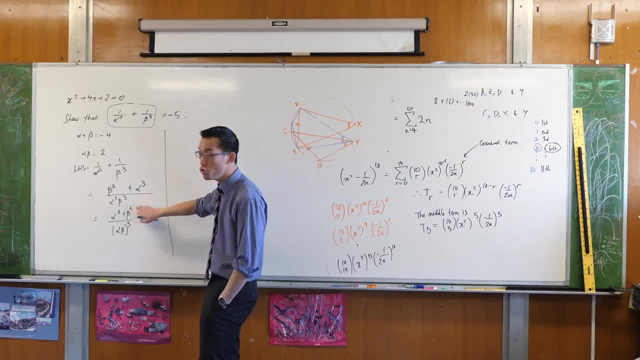 Now, as a two-unit student. in fact, you know an identity that can help you with this numerator. It's the sum of two things that have been cubed. So what's the sum of cubes' identity? Do you know it? 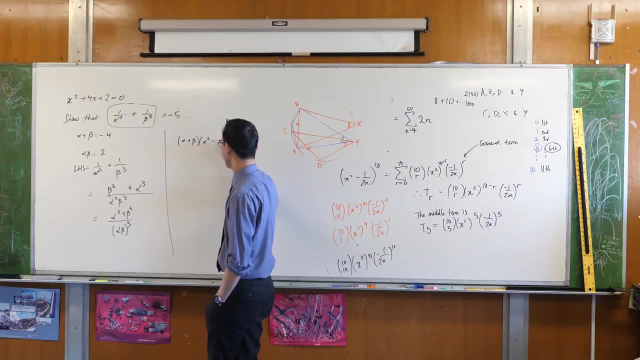 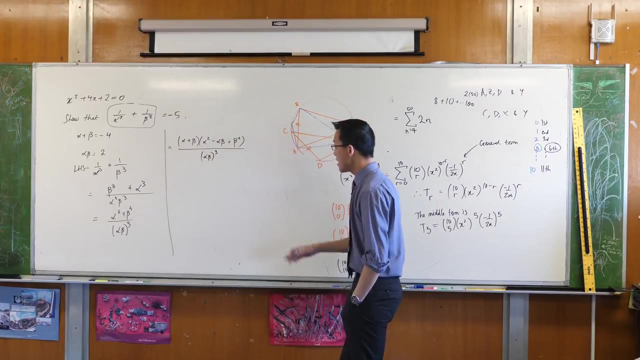 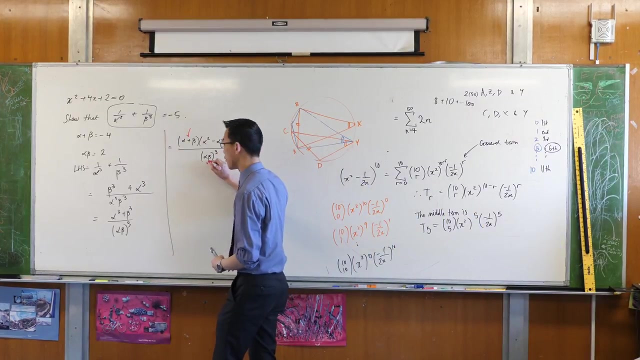 Yeah, Very good, Very good, Fantastic, And you've got this on your reference sheet, which is nice. So you've got this. Yep, it's on the reference sheet, Okay. So that's that. Okay. Now, this is really good, because I know what alpha plus beta is. I know what alpha beta is. 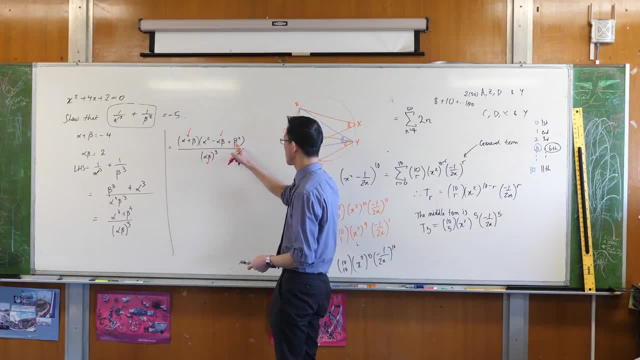 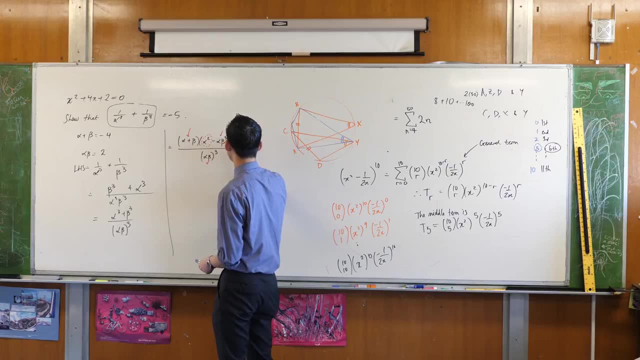 There's another alpha beta here, And so all that's left is: What do I do with this? these guys, okay Now. so what I'm doing is I'm trying to see through the question and notice: alright, these guys are the issue now, so I'm going to focus on those, okay. 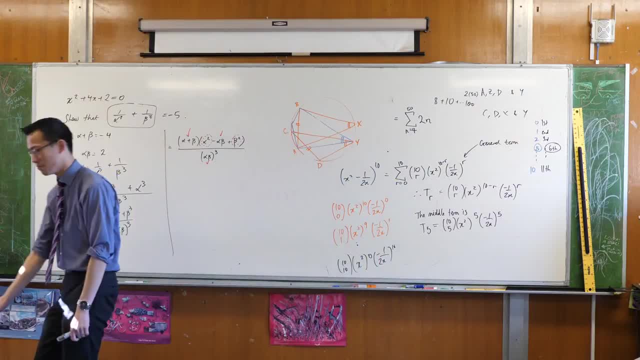 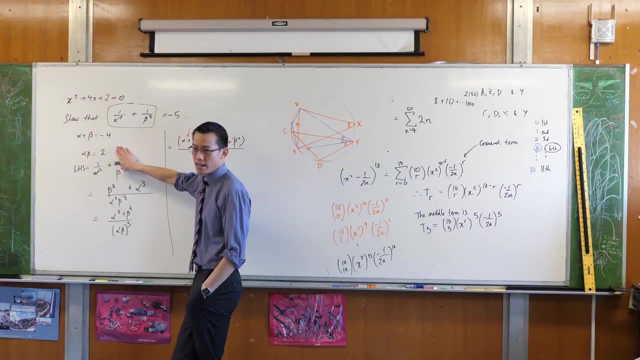 Now this bit takes a bit of fiddling. okay, To get an alpha squared and a beta squared. can you see that squaring this guy is not good enough, because the alpha squared and the beta squared will then be tangled up together. You'll get alpha squared times beta squared. 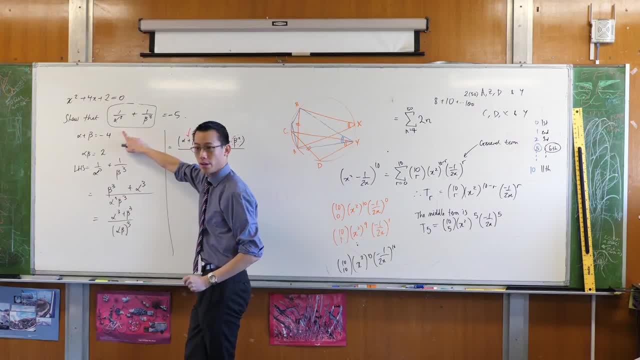 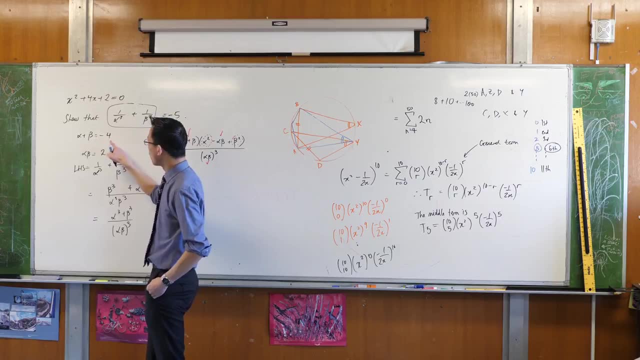 and you can't separate them. So, therefore, I'm going to have to do something with this guy, because they have the alpha and the beta separately. yes, So if I squared this on the left hand side, if I expand it all out, what would I get? 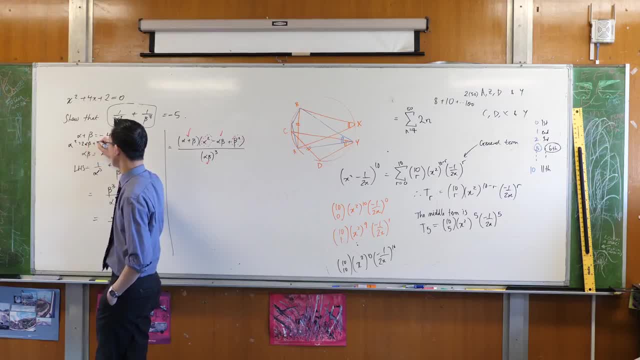 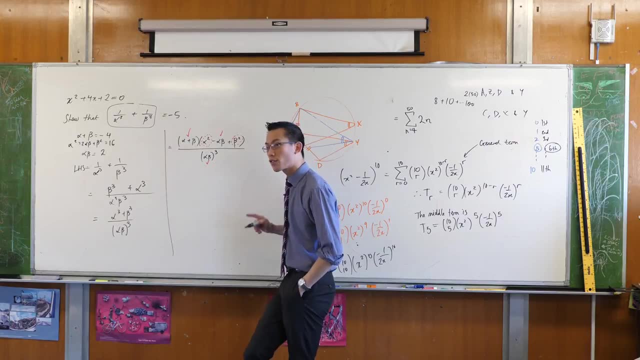 Alpha beta squared and beta. oh Yeah, alpha beta plus beta squared, do you agree? And that's 16, okay, Now I actually don't quite have that, but I've got something very close to that. watch this. 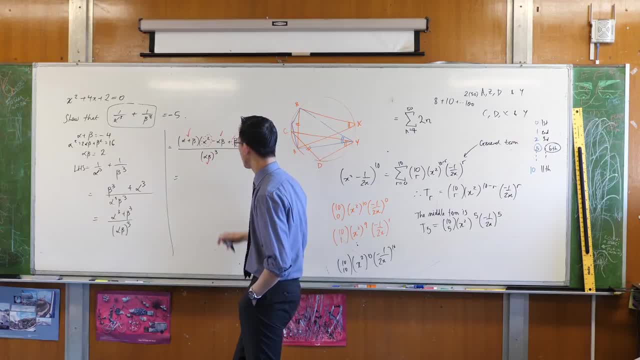 I'm going to subtract something. Yeah, I'm going to subtract something, So I'm going to do a two things in a row. I'm going to do a two things in a row, So I'm going to do a two things in a row. 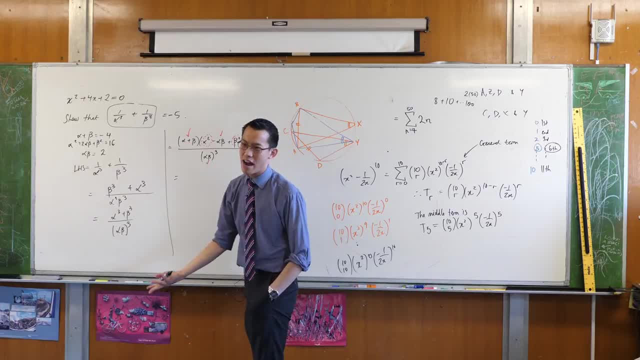 Well, so I'm going to replace one of those numbers. So the 문제 in this next line, the first thing I'm going to do is replace these guys. I don't need to keep writing them. I know what they are numerically. 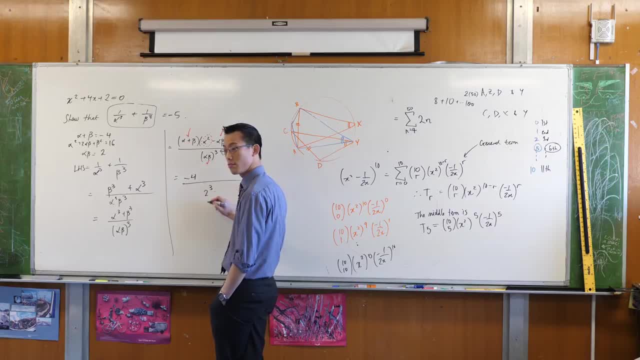 So that's negative 4.. On the denominator, I have 2 cubed. Is that okay? Now, what do I have in here? Well, I'm going to write this in terms of this: So it's alpha squared plus 2, alpha beta plus beta squared. I've done this because I know what. 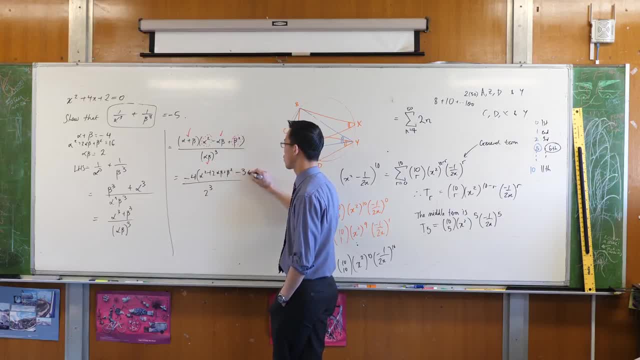 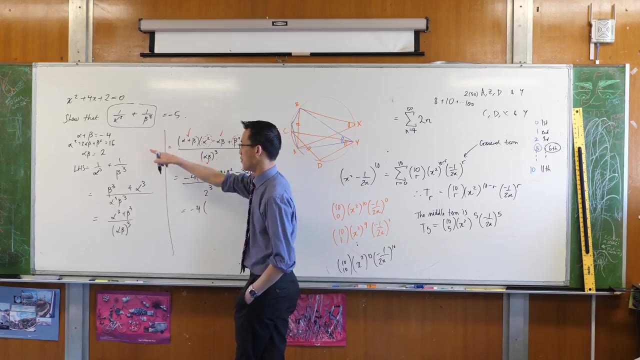 that's equal to, But this, of course, is not equal to what I wrote in the last line. To subtract 3 alpha beta. Is that okay? Sure enough, this does equal to that. I'm good, I'm pretty much there. So this is negative 4 times because I've written it over there. 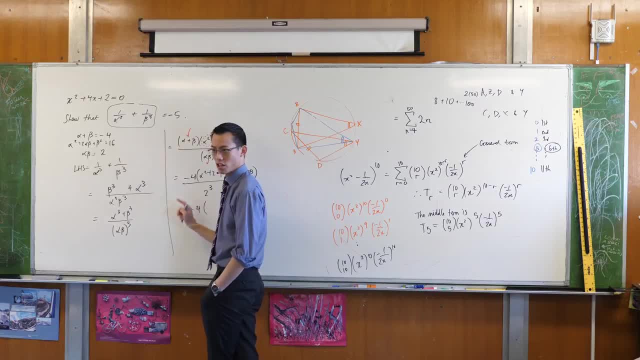 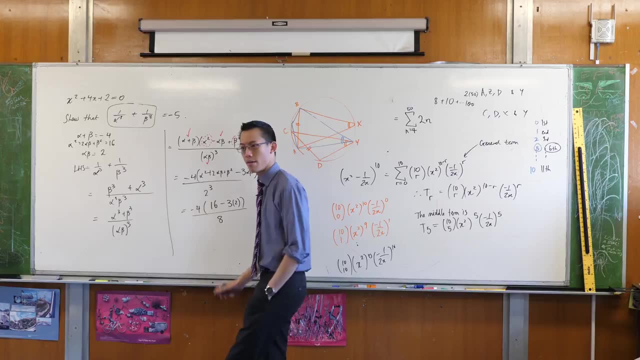 I can just substitute it for 16.. So if you write this down so you can refer to it, you're good. Minus 3 times what's that? 2. And then you're pretty much home and host. It is important. 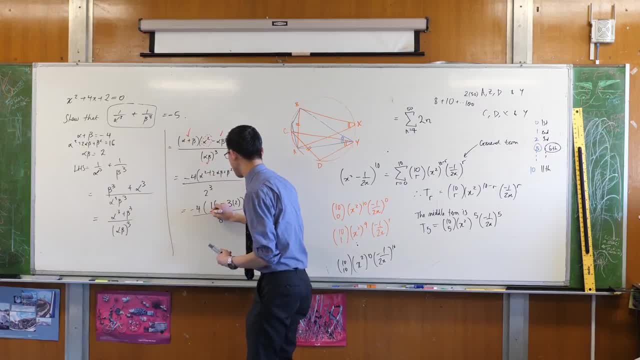 that in order to simply write down 16 here, I have to have written somewhere that alpha squared plus 2, alpha beta plus beta squared is equal to 16, just like I have here. If I hadn't have written this down I've got to show. probably my intervening line would. 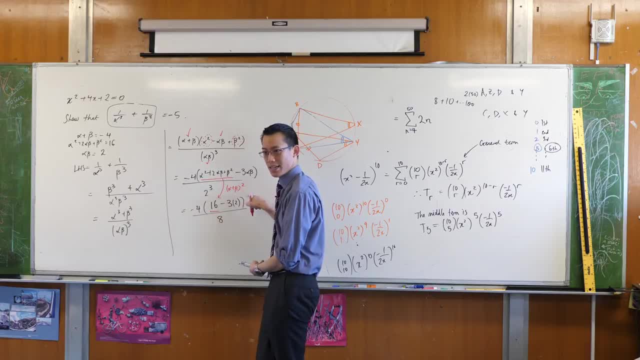 be this: I need to show. I recognise what that is because, remember, you know what this answer is going to be. so, therefore, just getting the number is not good enough. You actually have to show the steps the longest. It's the logic, the logic that gets you there.